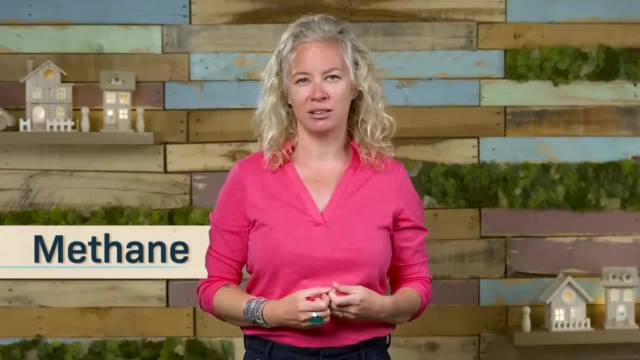 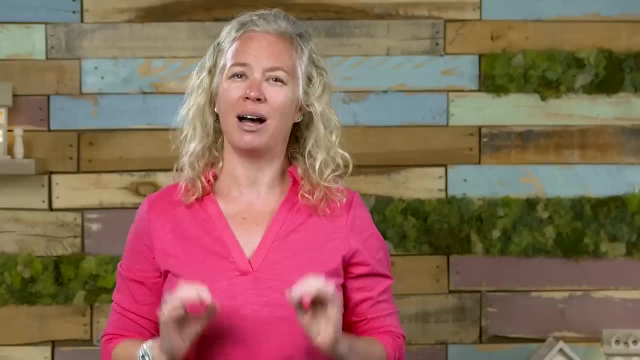 consists mostly of methane, one of the notorious greenhouse gases, And our means of extracting methane contributes to climate change, contaminates water and can even cause earthquakes. I'm talking about fracking. No, not the PG version of a cuss hollering and screaming. 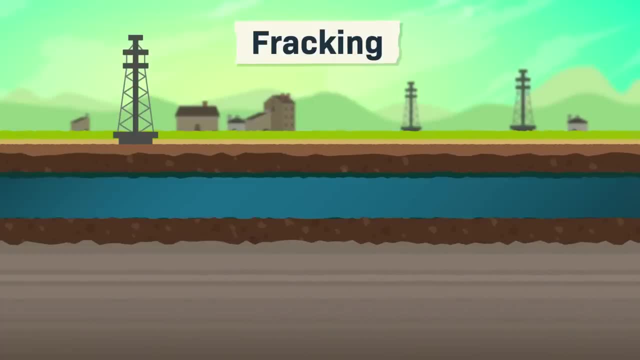 You heard when you stubbed your toe in front of your parents? Fracking is a way of extracting natural gas or crude oil from deep below Earth's surface. It uses high-pressure drilling and fluid to fracture underground rocks- hence the frack- and releases the gas within. But it also has some big side effects, Notably 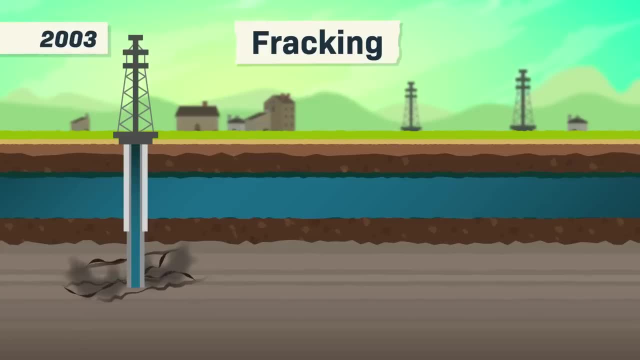 in 2003,, a new fracking method burst onto the scene just as the US natural gas supply was declining. By using mostly water instead of expensive gels and drilling not just down but also horizontally, this new method of fracking is becoming more and more commonplace in the US now. 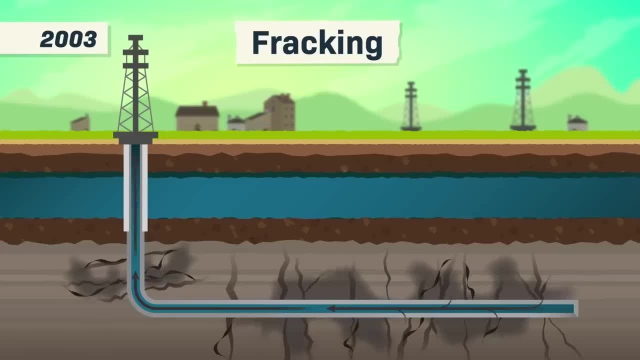 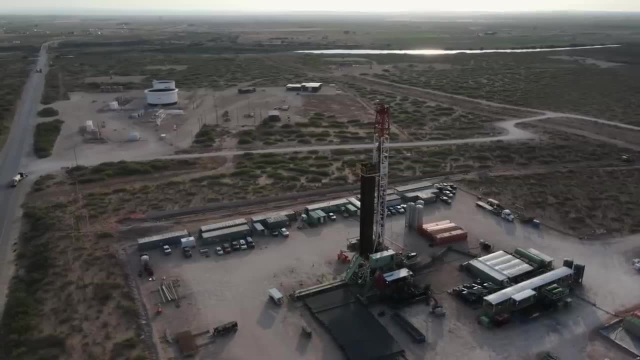 This new method made it possible to extract more natural gas than ever before, and more cheaply, from rock called shale. The fracking boom boosted the US economy. Extracting gas within US borders instead of importing it helped create 2.8 million jobs, and generate trillions of dollars in revenue Sounds like a net positive right, If only The downside is that extracting natural gas from shale is messy. Some methane inevitably escapes into the atmosphere. It'd be like whenever you sip soda from a straw. 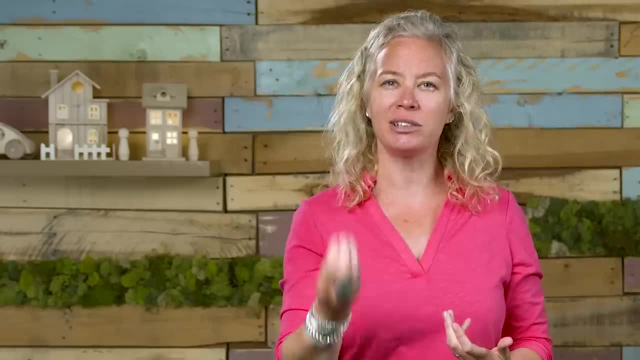 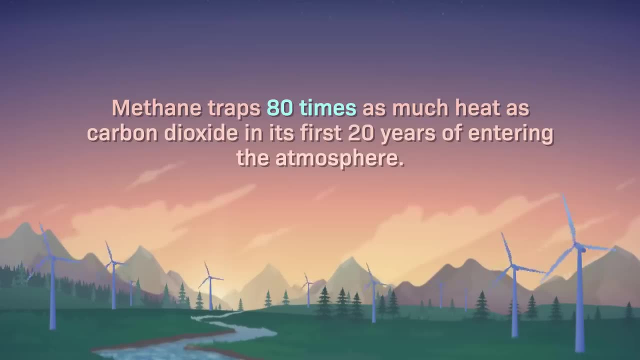 some of it came out the side of your mouth, Except here that soda is methane. This greenhouse gas traps 80 times as much heat as carbon dioxide in its first 20 years of entering the atmosphere. Global methane levels have spiked since 2007.. 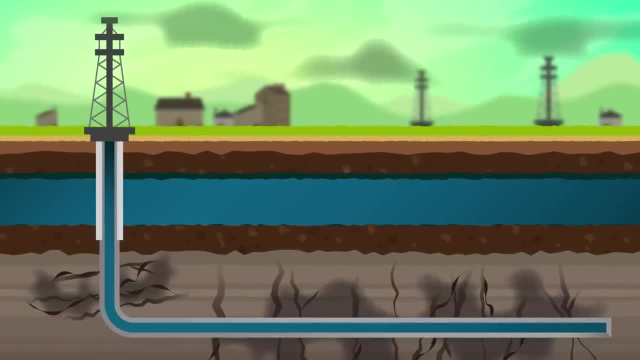 The fracking boom, which has since spread beyond the US, is a prime suspect in that whodunit. Another problem: Use of fracking wells keep releasing methane even if they don't get plugged up, which costs millions of dollars and doesn't always happen To make matters even. 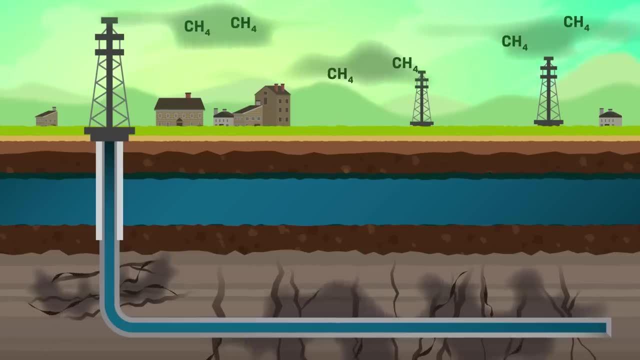 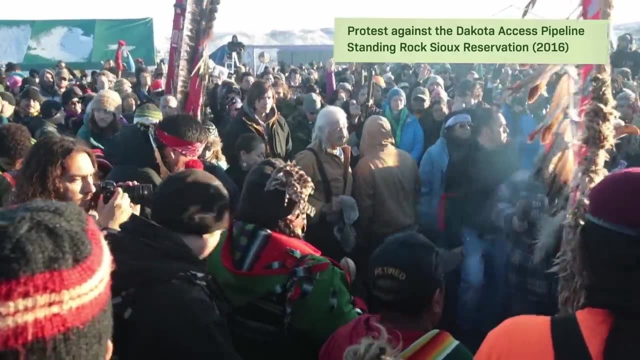 worse, pipelines transporting oil and natural gas from fracking sites leak, which can threaten nearby communities. For instance, the Standing Rock Sioux Tribe protested the construction of the Dakota Access Pipeline, which was built in 2017 and today runs directly beneath one of the 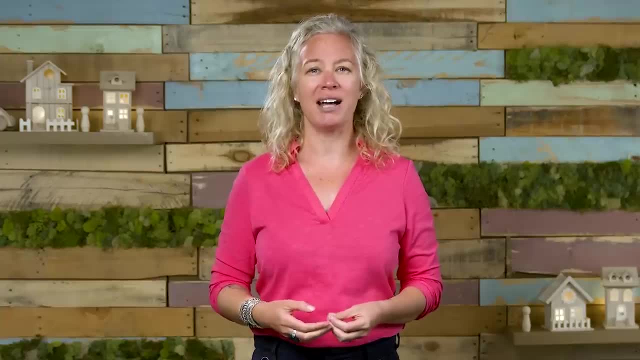 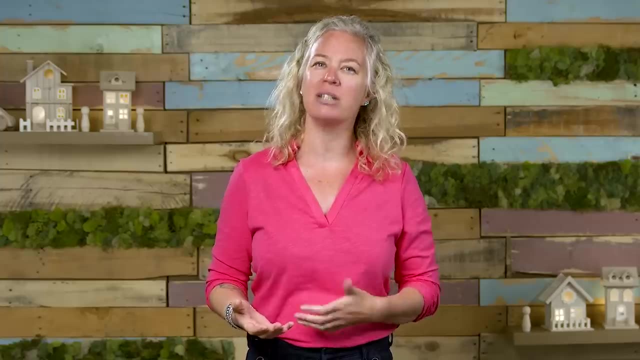 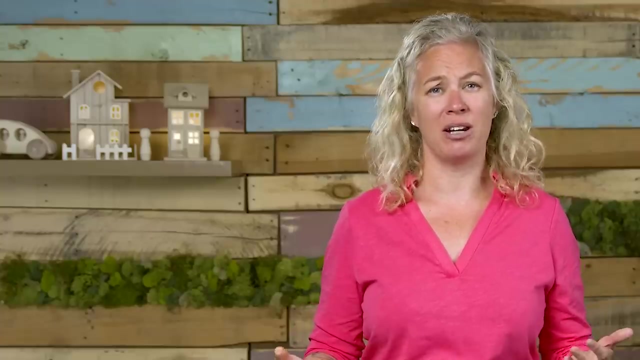 reservation's main water sources. So overall, natural gas is a major energy source, But it will also likely play a big part in decarbonizing energy worldwide. Burning natural gas actually releases significantly less carbon than burning other fossil fuels, And burning it to generate electricity or heat makes less air pollution than something like coal. 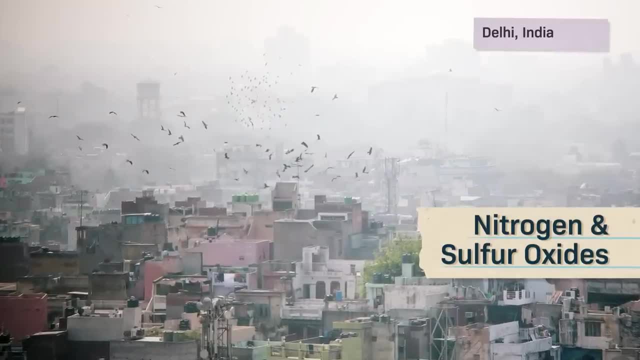 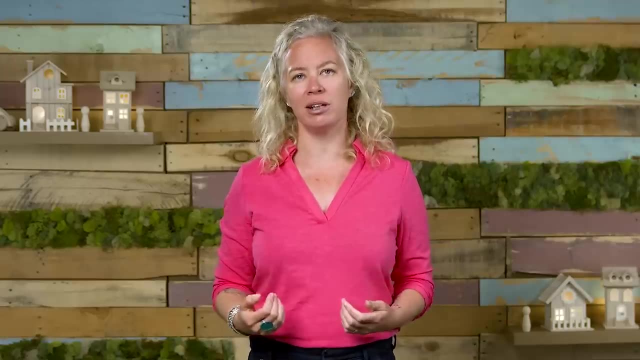 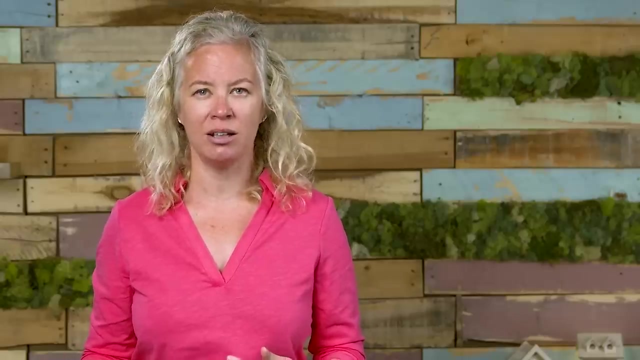 It also releases fewer pollutants like nitrogen and sulfur oxides—pollutants that contribute to unhealthy air quality and form smog and acid rain. But not everybody has the luxury of clean air and lower pollution energy. Millions of people in low-income countries don't have access to natural gas, So they depend on 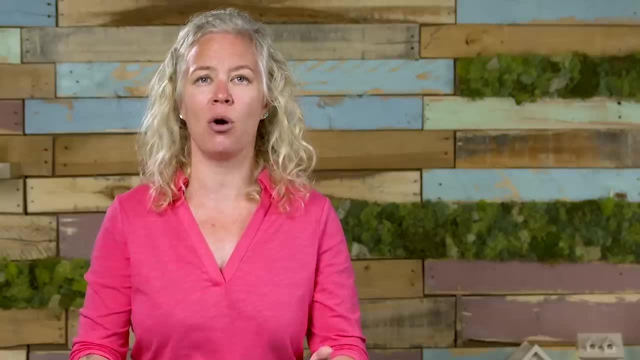 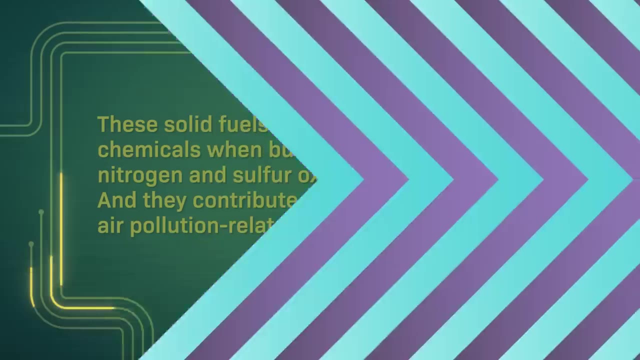 high-polluting solid fuels to heat their homes and cook dinner, such as coal or biomass. Biomass includes materials such as charcoal or wood or dung from livestock. These solid fuels release harmful chemicals when burned, including the nitrogen and sulfur oxides that make smog. 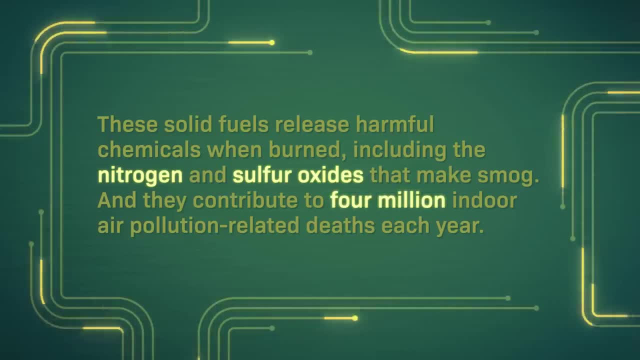 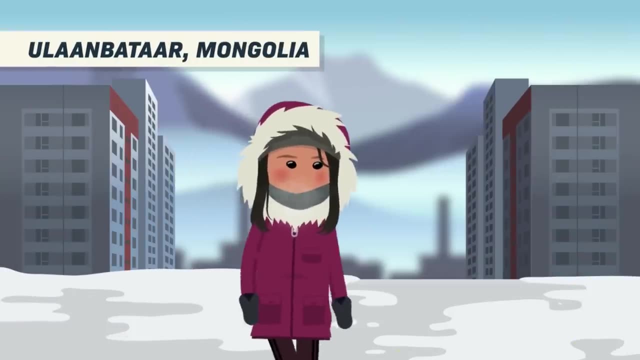 And they contribute to 4 million indoor air pollution-related deaths each year. Let's head to the Thought Bubble. Take a wintertime stroll through Ulaanbaatar, the capital city of Mongolia, and you'll notice the chill doesn't just nip your nose, It mauls it. 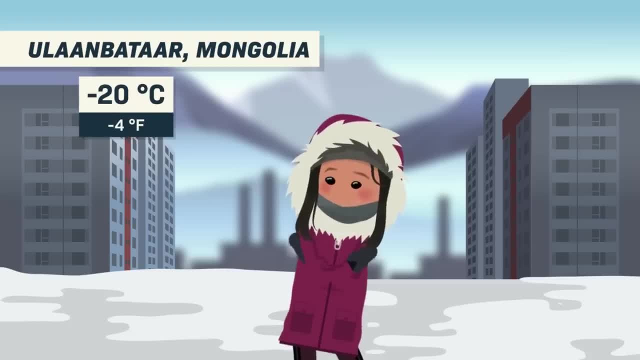 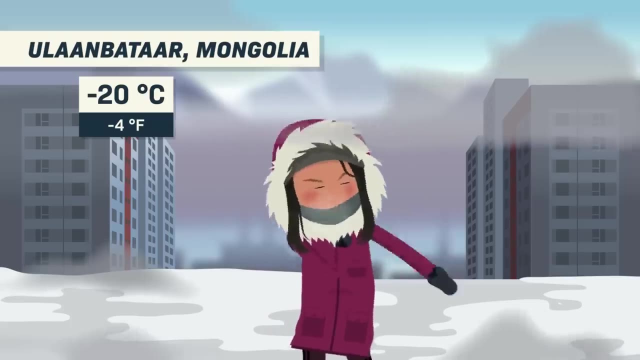 with an average January temperature of negative 20 degrees Celsius. Ooh, delightful, I love the cold. But before your nose goes numb, you'll notice the sting in your throat. A thick smog hangs over the city, trapped at ground level by cold winter air and surrounding mountains. That smog is full of teeny-tiny soot. 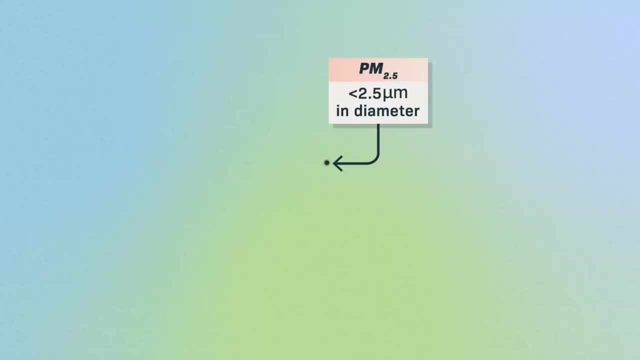 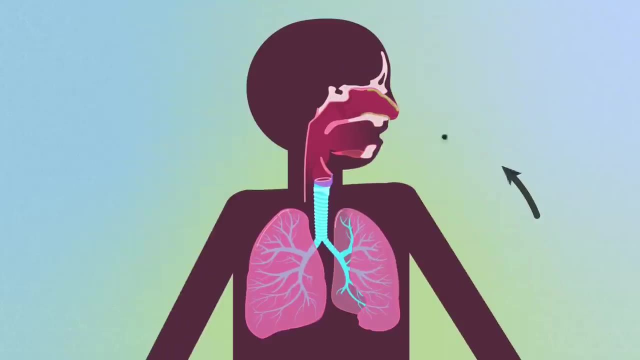 particles called PM2.5.. These tiniest of polluting particles are 30 times smaller in diameter than a single strand of human hair, But they pack a mean punch. When someone breathes them in and these particles get lodged deep in the lungs and bloodstream, they can cause pneumonia and 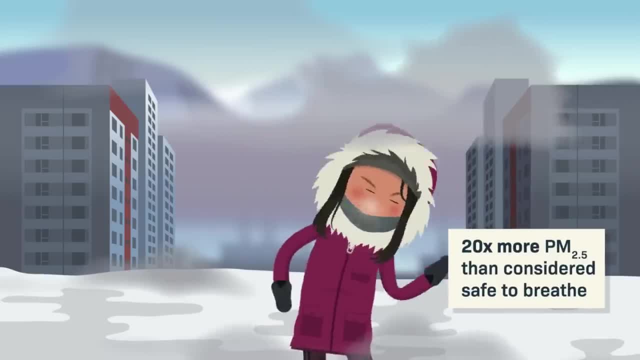 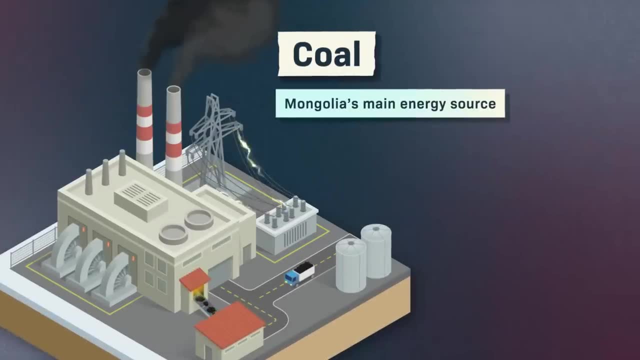 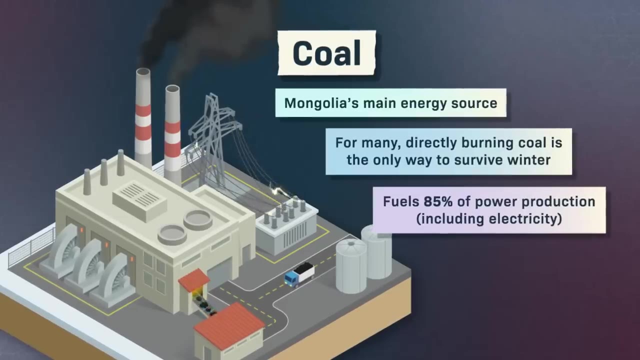 bronchitis, And Ulaanbaatar's air can carry 20 times more of these particles than what's considered safe to breathe. Coal is to blame here, Mongolia's main energy source. For many households, directly burning coal is the only way to survive winter, And coal fuels 85% of the country's power. 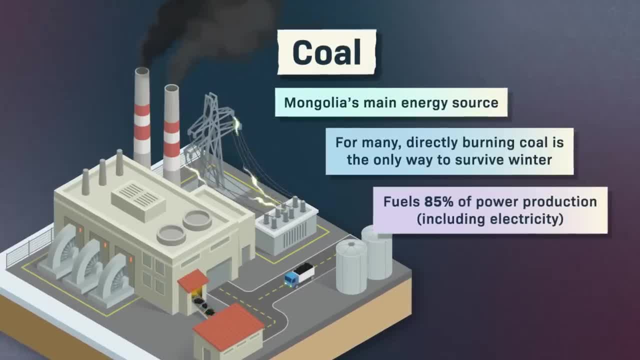 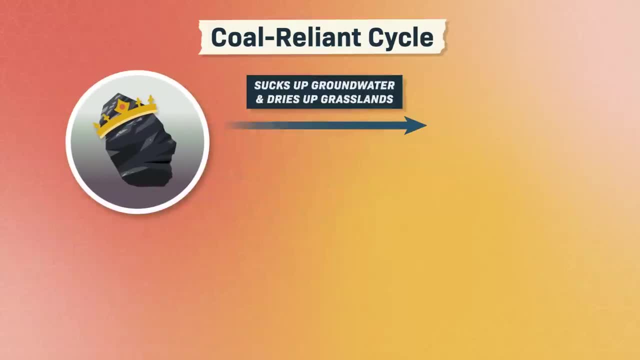 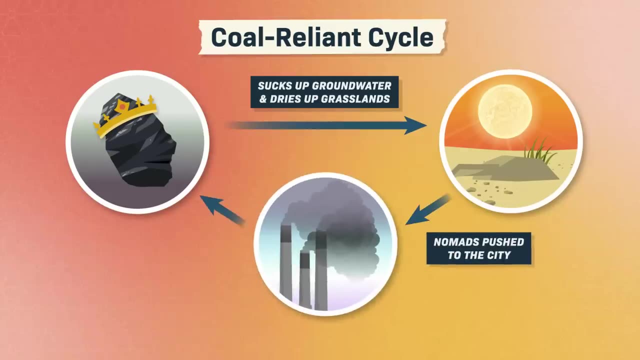 production, so even electricity runs on it. Ultimately, Ulaanbaatar finds itself in a coal-reliance cycle. Demand for coal drives more coal mining, which sucks up groundwater and dries grasslands to a crisp. As grasslands disappear, nomads are pushed to the city And 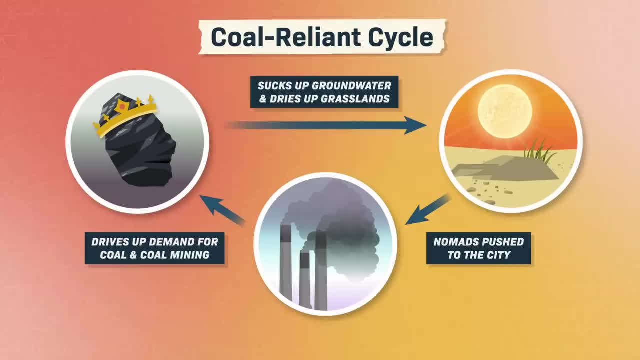 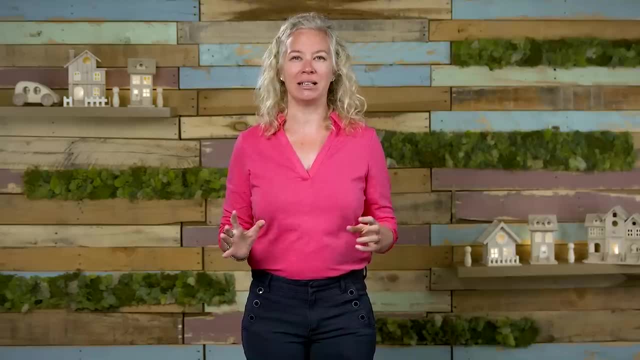 there they join the masses dependent on coal to stay warm, which drives more demand for more coal. Thanks Thought Bubble. Stuck. in a loop like this, breaking up with coal won't be easy. Even replacing coal stoves with coal-fueled electricity just pushes the problem farther. 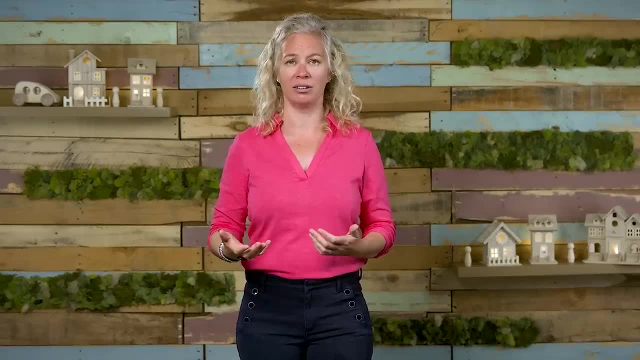 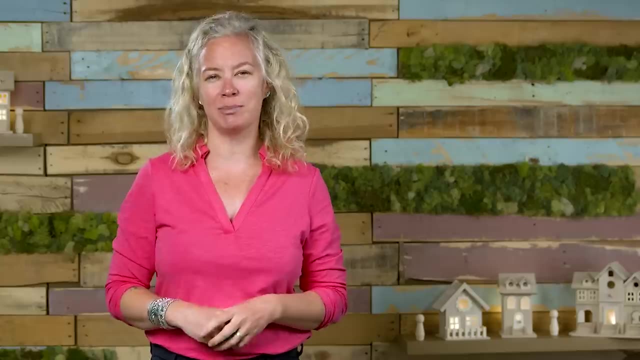 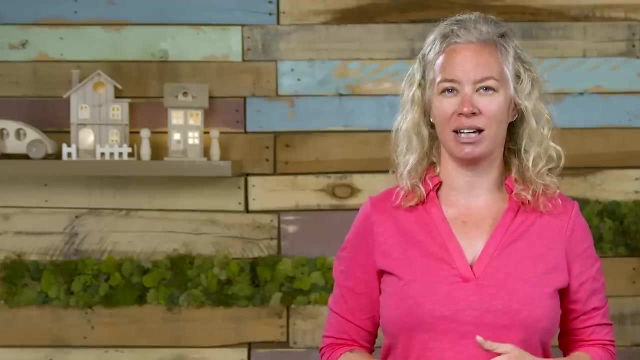 up the hill Like passing a sizzling ember from one hand to another. Ow When it comes to reducing carbon emissions and making our world a cleaner place for everyone. the situation is messy, and heating is no exception. Increasing access to natural gas might help Ulaanbaatar and other cities like it. 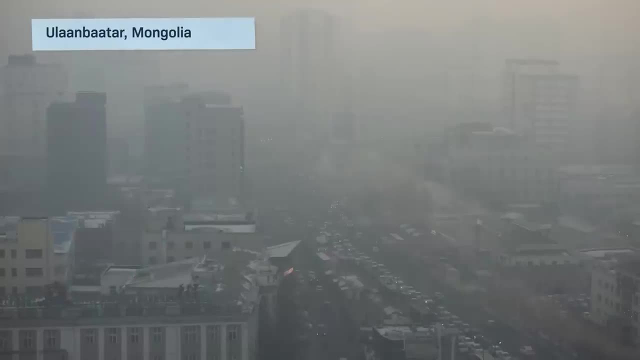 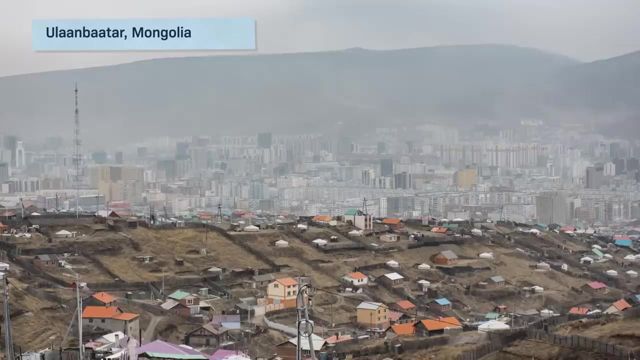 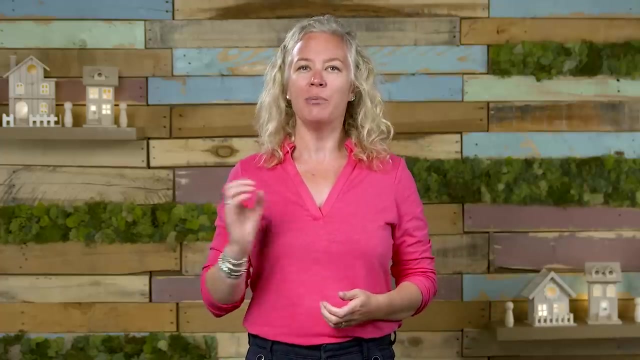 but it's still a very complicated solution And, as long as electricity runs on coal, bringing electric heaters to more people won't be enough to see cities like this out of the smog or to see our planet out of rising emissions. Renewable energy like solar or wind power would definitely help with this, But there's 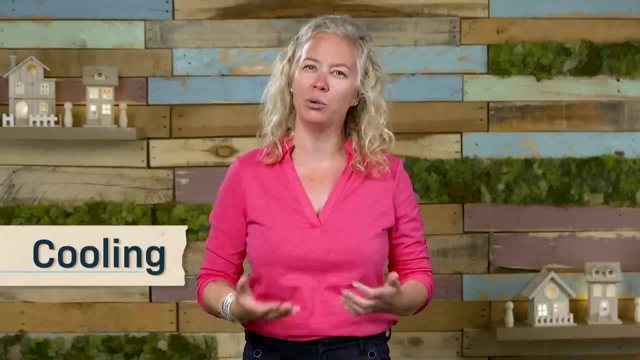 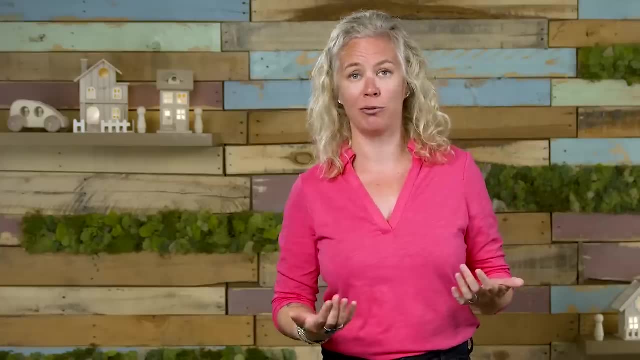 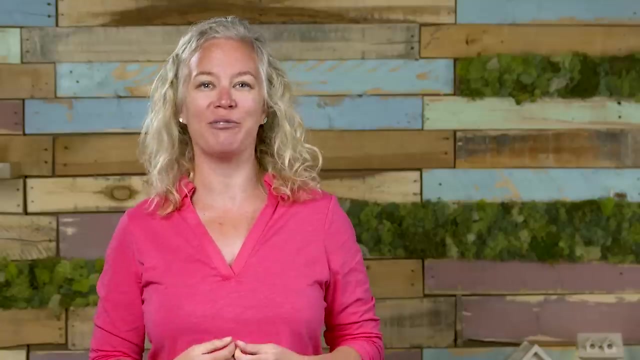 still another side of the equation we haven't talked about yet: Cooling. Quick guess what's on track to be the most energy-consuming appliance in my house. Based on my current rate of waffle consumption, it feels like it should be Maybe a waffle maker, but actually it's my air conditioner. Back to my love of frigid. 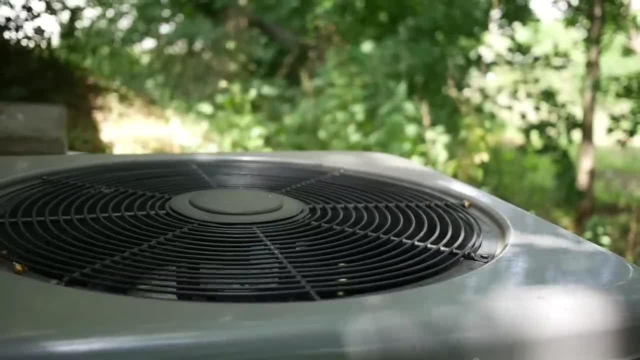 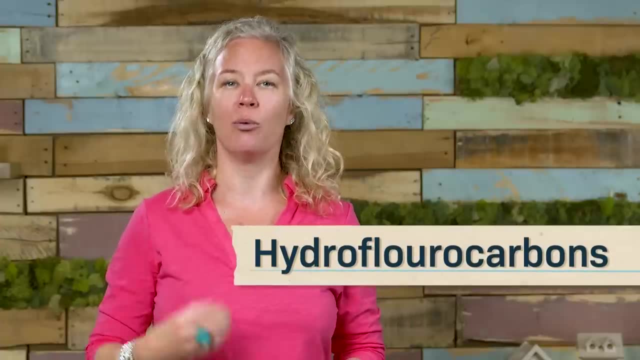 temperatures. Air conditioners are heavy electricity consumers and it's mostly fossil fuels powering that electricity. Air conditioners also have a nasty way of releasing hydrofluorocarbons, one of the greenhouse gases with the longest name and the most powerful global warming. 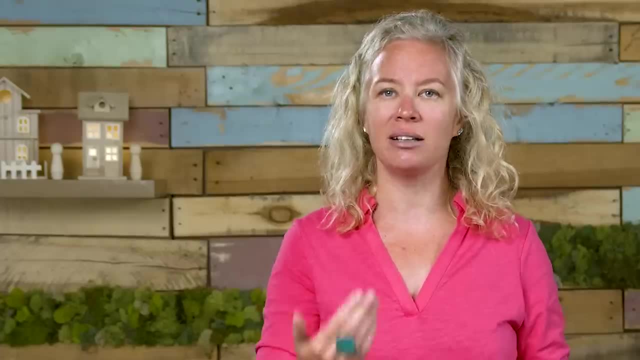 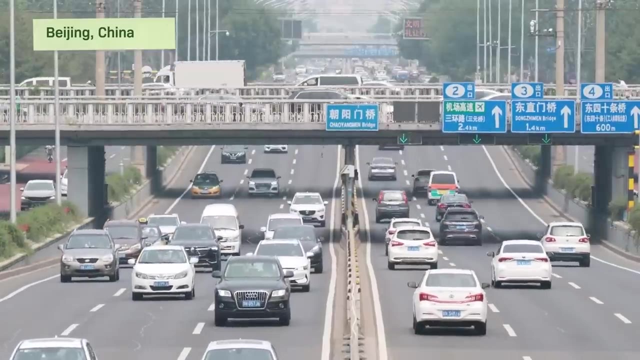 abilities, But we can't just ditch the ACL together. As the climate warms, the need for air conditioning rises too. Billions of people are facing global warming's deadly climate. We are doing more than just headliest effects, including more frequent severe heat waves. 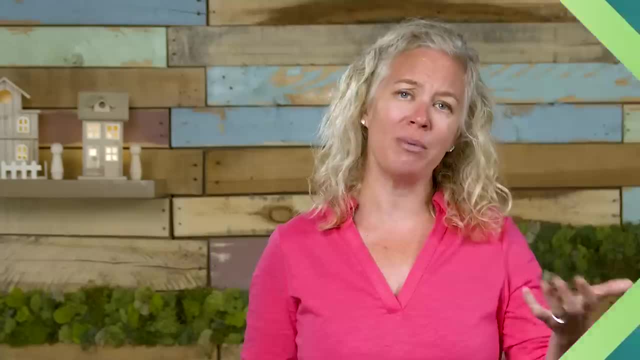 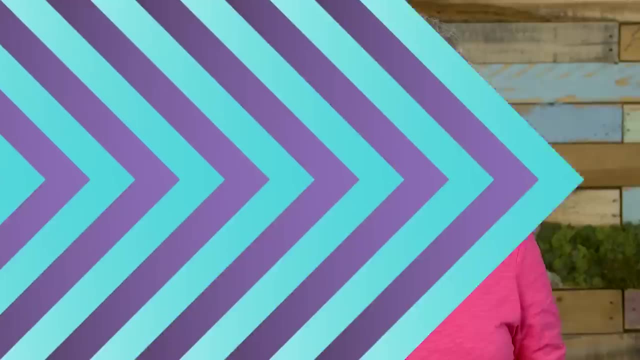 To some, air conditioning becomes a life-or-death necessity. The problem is, it's a necessity that millions of people can't afford. so it's also an issue of justice and equity. And, to make things more complicated, the same air conditioning that helps people survive. 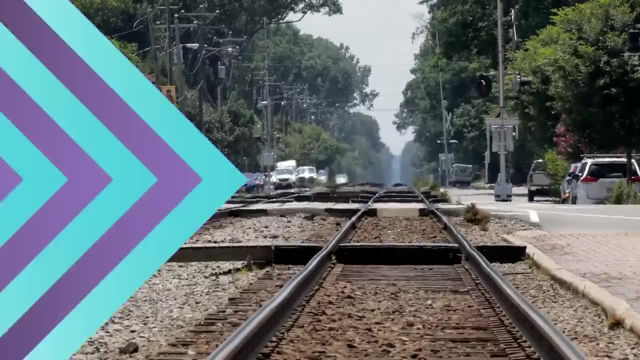 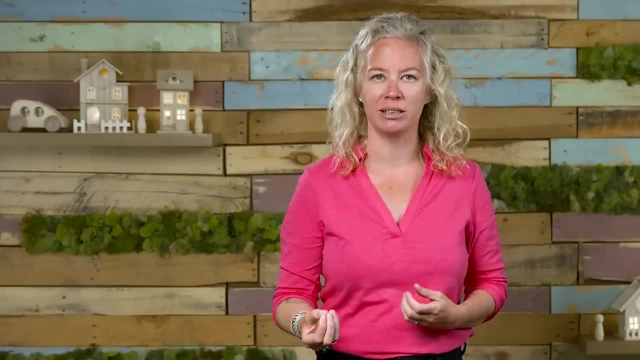 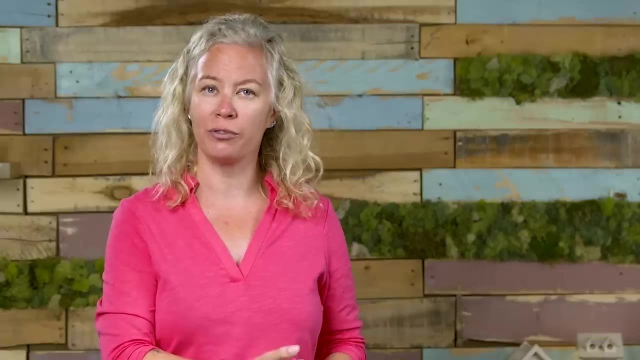 blazing heat also exacerbates those conditions in the first place, But it doesn't have to be that way. One thing governments can do is raise the minimum efficiency requirements for appliances so that any new AC unit has to meet a certain standard, Moving away from hydrofluorocarbons and towards refrigerants with lower greenhouse warming. 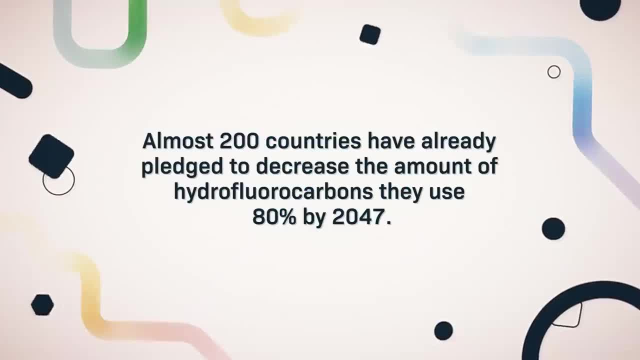 potential would also help reduce emissions And in fact, almost 200 countries have already pledged to decrease the amount of hydrofluorocarbons they use- 80%- by 2047.. Besides improving existing air conditioner designs and scaling up carbon-free electric, 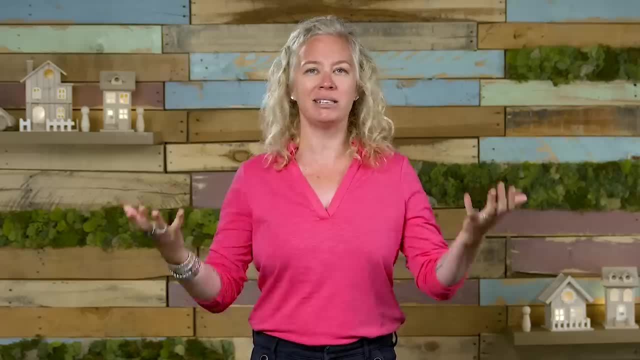 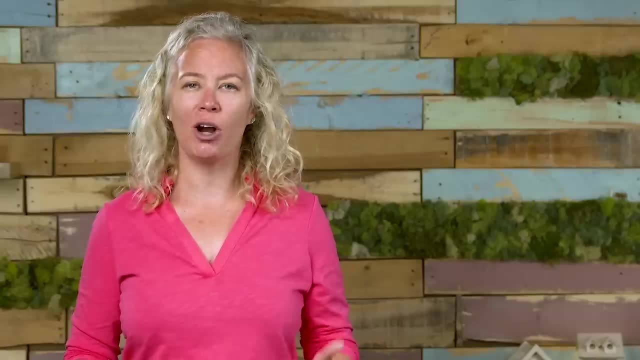 electricity sources. another option to cool our homes is to ditch AC units altogether and consider other technologies. And, as a big bonus, these solutions could help us with decarbonizing heating too, and even help us move away from natural gas. Take the heat pump. 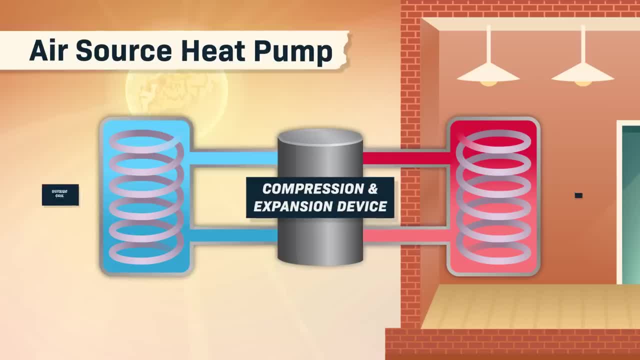 Heat pumps use the same basic mechanism of an air conditioner. When it's warm out, both heat pumps and AC units use heat-absorbing liquids, called refrigerants, to move heat outside, so your bedroom stays cool. But heat pumps can also do the opposite. 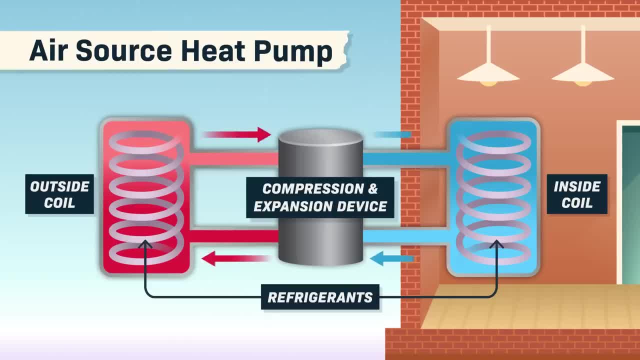 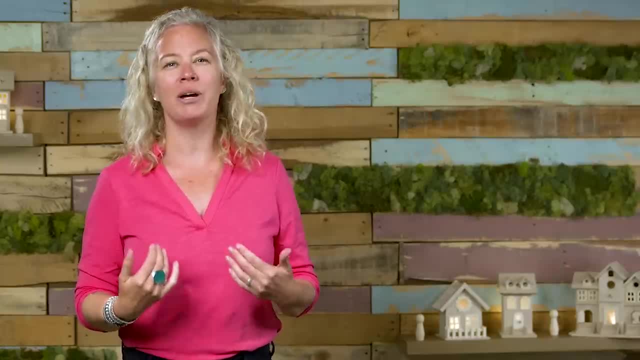 In the winter they can bring in heat from the cold air outdoors to keep your home warm. That might sound weird, I know. when I'm out waiting for the bus in January here in the Northern Hemisphere, my first thought isn't: oh, there's so much heat in the air right now. 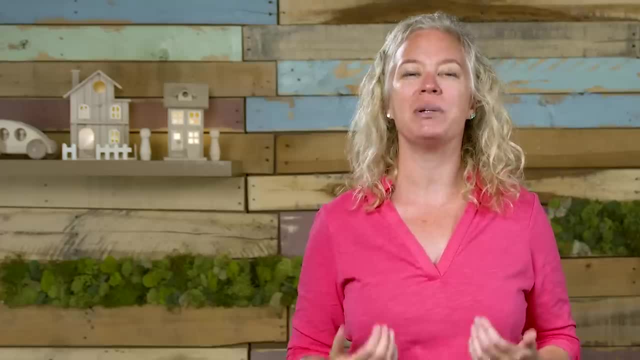 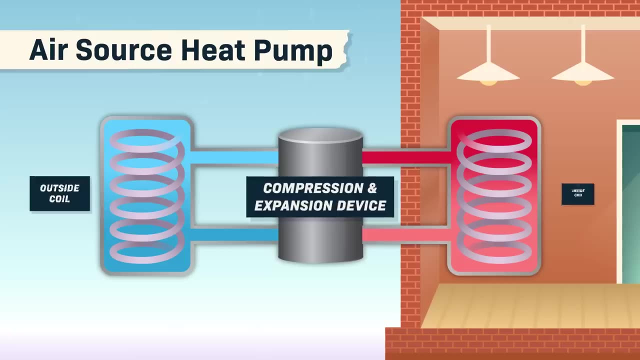 But for as cold as winter is, the refrigerant in a heat pump is even colder. It can get down to negative 50 degrees Celsius depending on the model. So the refrigerant absorbs and concentrates the little bit of heat linked to the air. 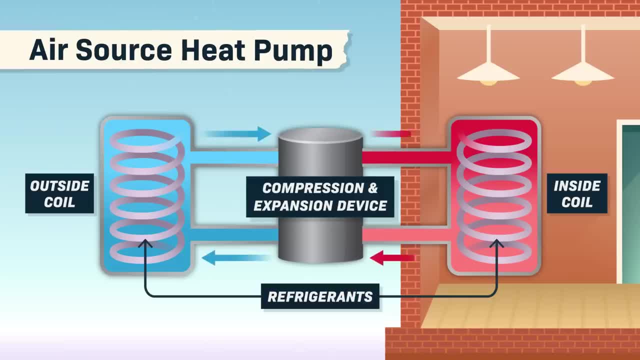 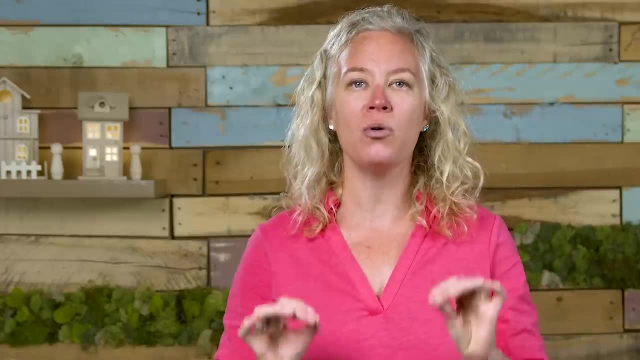 And when it's hot, the heat turns it into a gas. This refrigerant gas is then brought inside and pressurized into a warmer gas so that it can transfer the sweet, sweet warmth of the air in your house. When powered by carbon-free electricity, heat pumps emit almost no greenhouse gases. 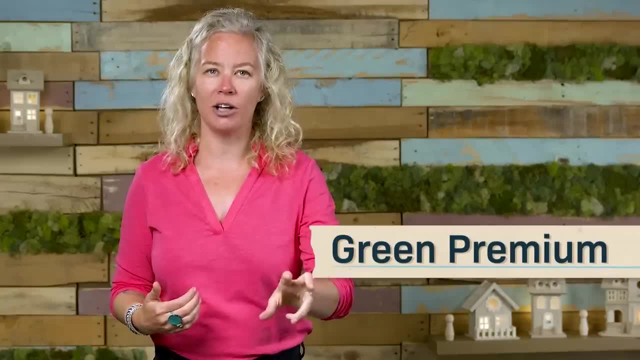 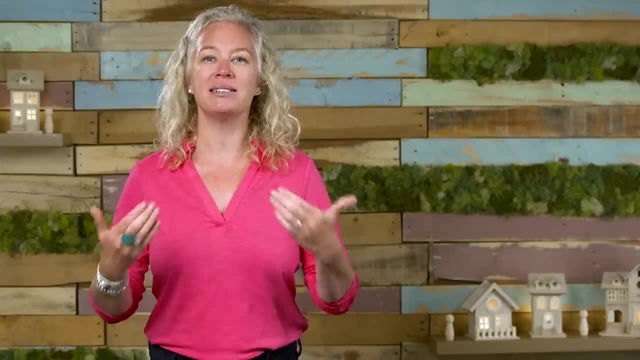 And they can even have a negative green premium. That's the cost difference between an energy source that releases carbon and one that doesn't. A negative premium Means that in some places it's already cheaper in the long run to install a heat pump than 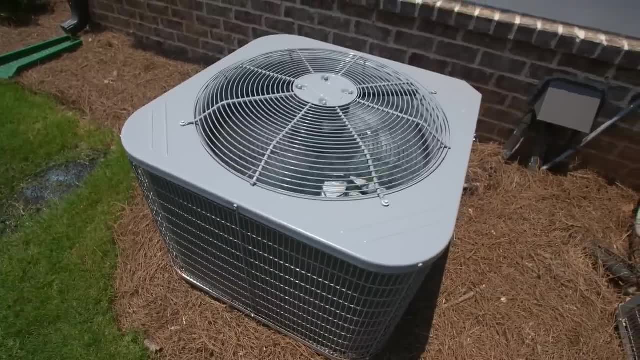 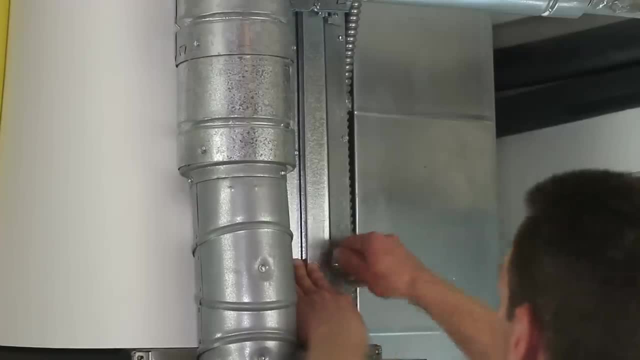 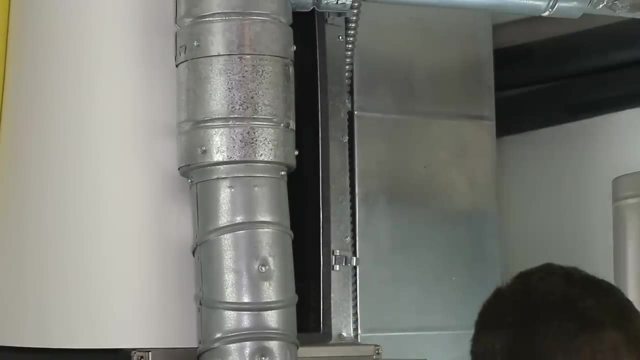 to run a natural gas furnace. That said, one barrier to heat pumps is that AC units and natural gas furnaces last a long time. It's up to individual homeowners and building developers to install heat pumps in the first place, And if my very expensive furnace is still kicking, it would be hard for me to get excited. 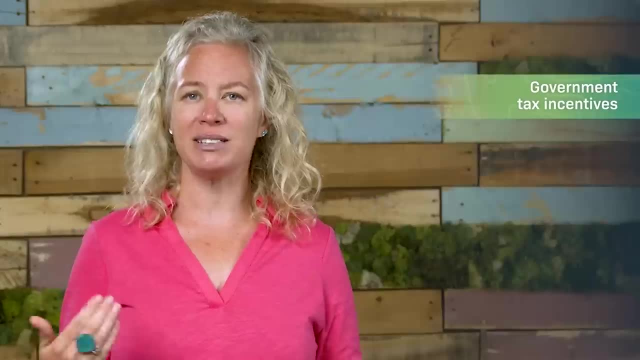 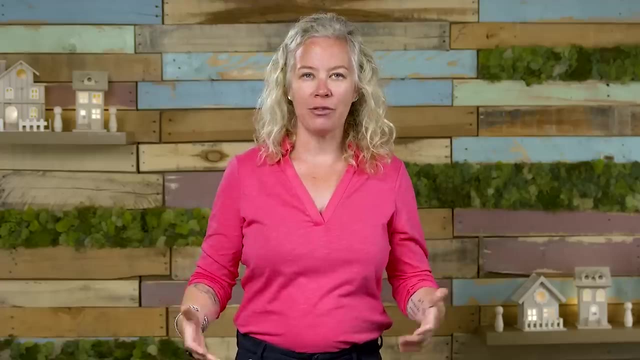 about forking over the cash to replace it with a heat pump. Enforcement tax incentives and loosening building codes could be one way of encouraging more people to make the switch. But a third path to decarbonization is to work with the systems we've got and find. 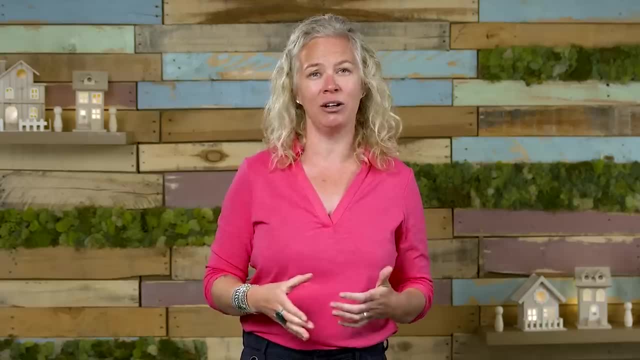 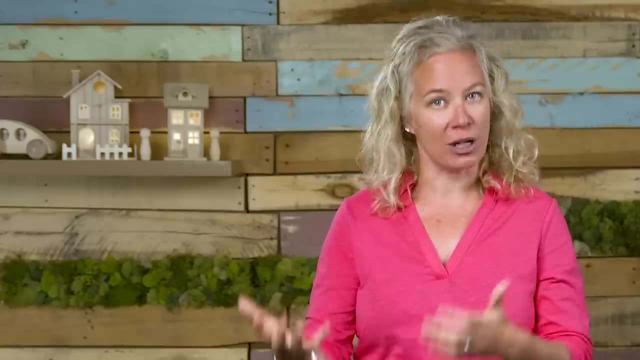 new ways of powering them, And for heating in particular, there's a lot of options. My favorite: Trash. Now, unless you're me or a raccoon, it might seem like not much good can come out of a steaming pile of trash. 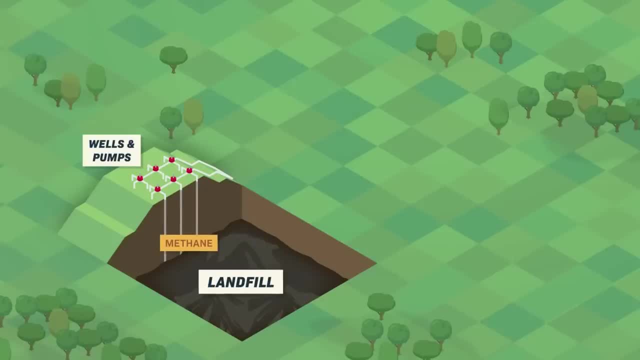 But the trash heaps in our landfills already release gases. they decompose. released gases. they decompose and that gas can be captured, converted and become a low-emission replacement for natural gas in our existing furnaces. Renewable drop-in fuels can also help. 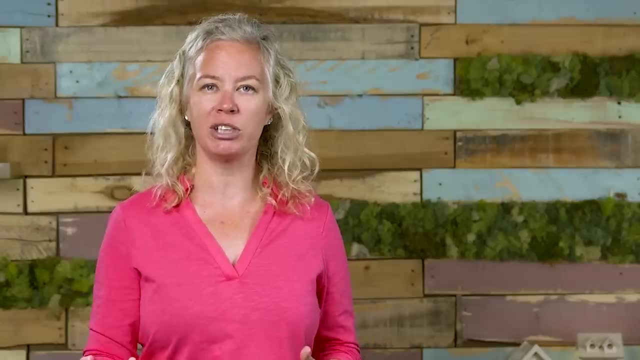 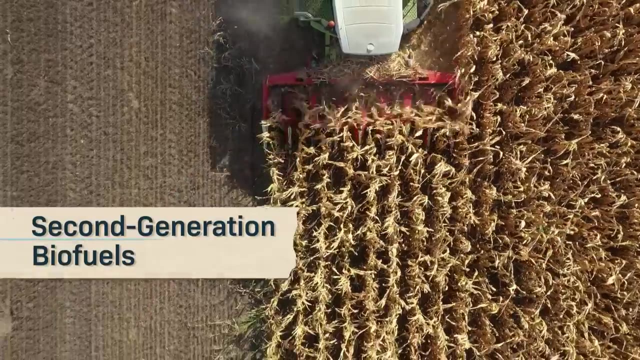 taper off emissions. These are basically fossil fuel substitutes made from renewable materials, and they can step in for natural gas in our heating systems. For example, second generation biofuels can be made from non-edible crops that are already being produced alongside our food. 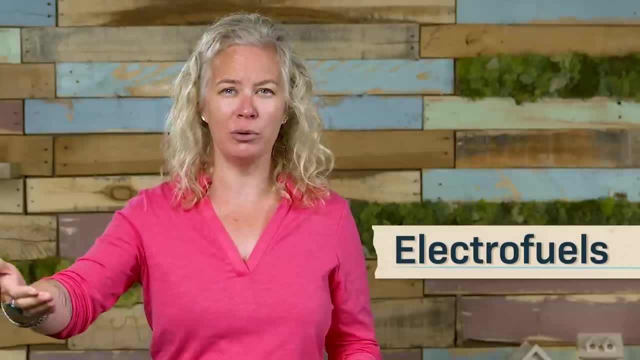 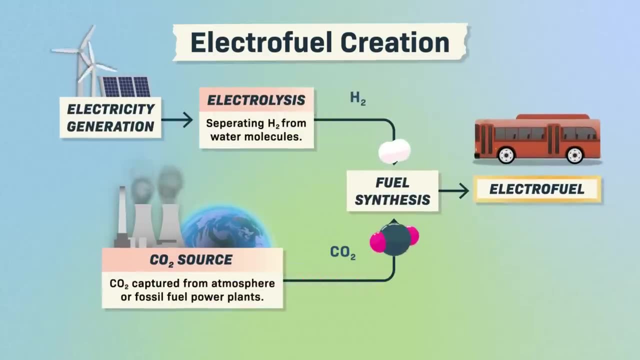 such as straw and corn husks. Meanwhile, electrofuels go a step further by not requiring crops at all. They're made by capturing carbon dioxide and mixing it with the hydrogen from water molecules to create some of the same molecules found in fossil fuels. Since 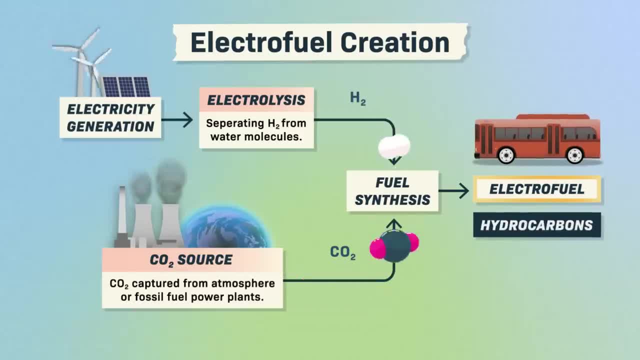 electrofuels are made of hydrocarbons just like traditional fossil fuels. burning them would release carbon dioxide, But because that carbon was just captured from the atmosphere or from a fossil fuel power plant, we wouldn't be adding any new emissions to the atmosphere. 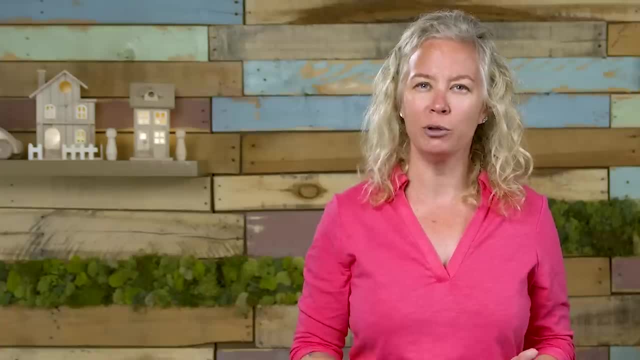 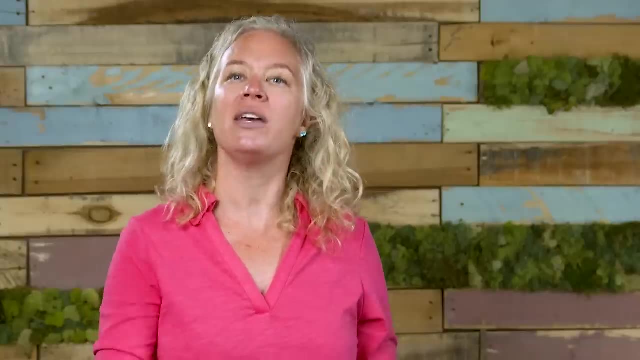 Then there's the challenge of that pesky green premium. These drop-in fuels can also carry a high up-front cost compared to fossil fuel energy. By offering a renewable alternative, they can help us reduce emissions as we wean our heating systems off the fuels they were built for. 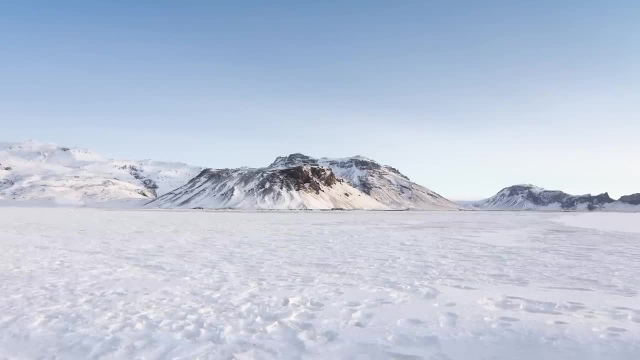 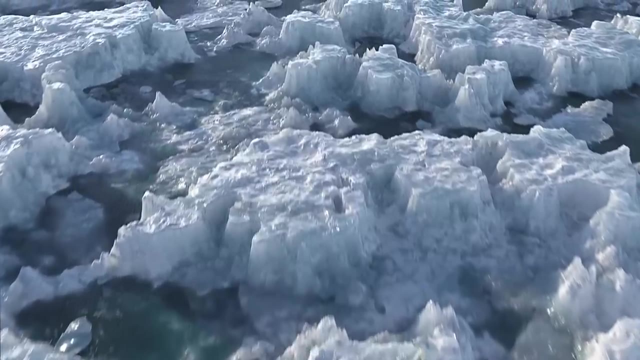 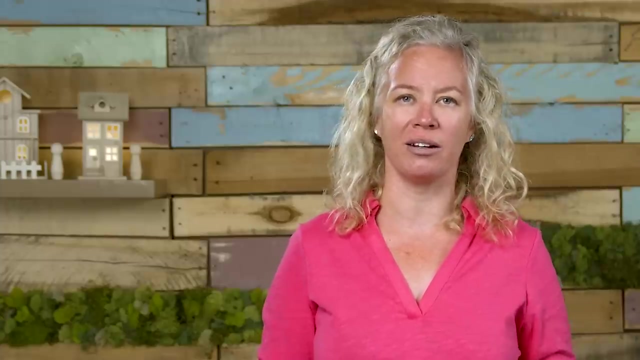 Humans have devised ingenious ways of keeping warm and staying cool everywhere, from the Arctic Circle to the Mojave Desert. Unfortunately, some of those energy choices have helped bring us to our current mess- the climate crisis- But that's safe. Same ingenuity can help us tackle the road ahead.